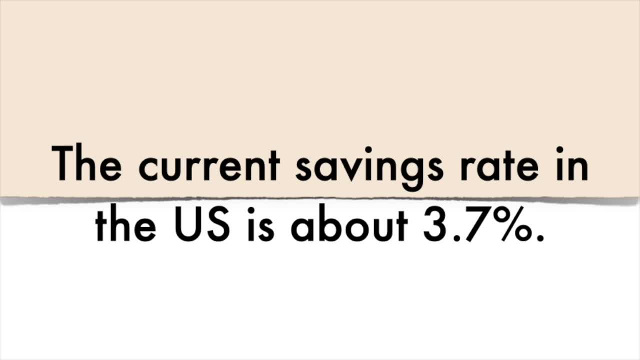 as of 2020, and this looks at savings of disposable income, not gross or take-home, which may be even lower. I am very surprised by these numbers and it's probably because I'm engrossed in the fire community, where savings rates are 10x this number. but get this the personal savings rate for. 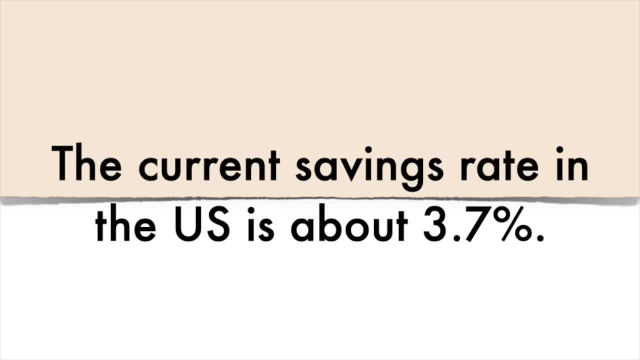 Americans peaked in 2020, when US households saved, on average of over 15 percent of their income due to COVID. The spread of COVID limited the ability for all of us to go out and spend our money, which resulted in being able to save more than usual. but, as we all know, things shifted back. 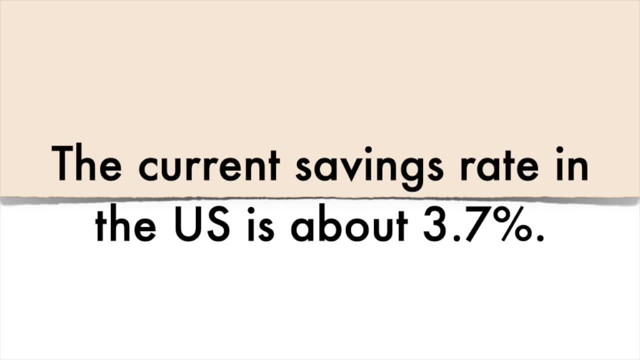 but this was a light bulb moment for my husband and I. What this showed me is that if my husband and I could wrangle in our consumerism ways, we could increase our savings. During COVID we started to build our savings because we finally could. We were forced to because of 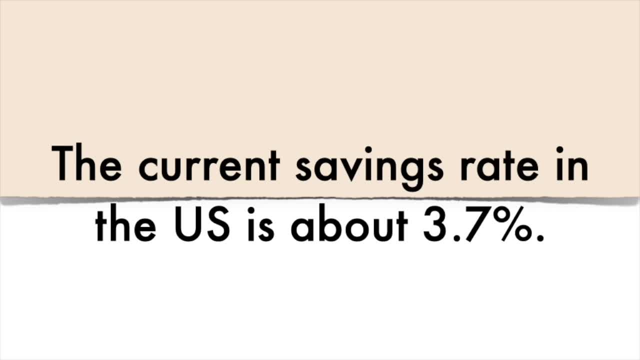 the circumstances and we began to build money-saving habits that stayed, but before COVID we were not living. We were living paycheck-to-paycheck per se, but we were saving less than we could and we were not sticking to a consistent savings rate. We were investing. we had some cash in our bank accounts. 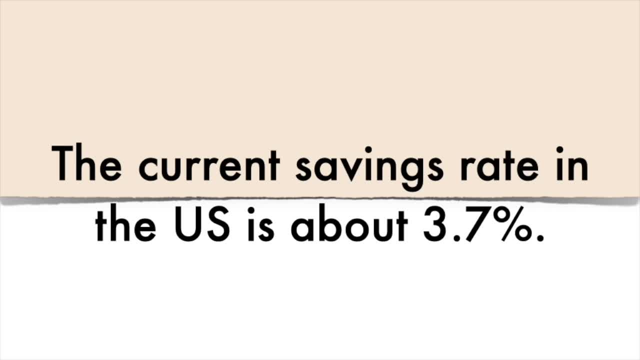 but we didn't have a clear direction or clear target to focus on. We could have been doing much more when it came to savings. One of the biggest mistakes we made on our FI journey was not tracking our savings rate sooner and not understanding the value of cash in our total 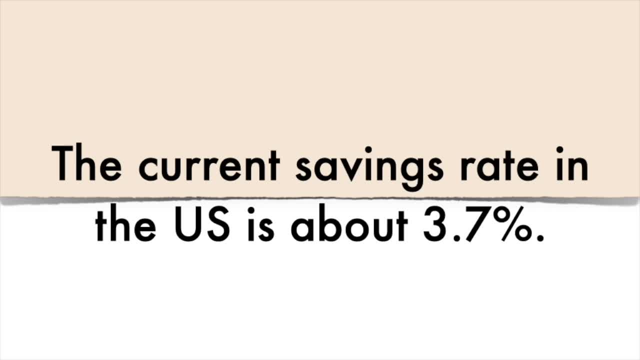 portfolio, not only for emergencies, but for security and a peace of mind. Savings helped us get out of the paycheck-to-paycheck cycle and we were able to save a lot of money. We were able to build a financial mindset that helped us truly begin our FI journey. So here's the average savings: 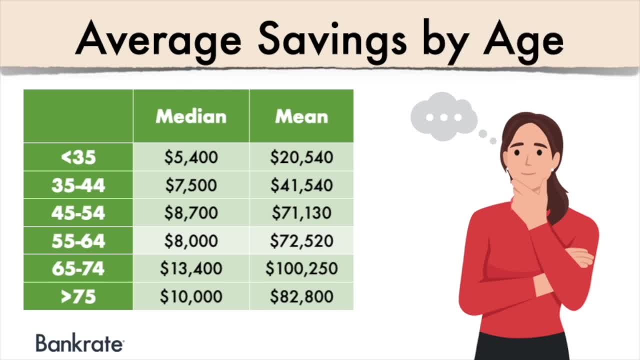 account balance by age, according to the Federal Reserve's Survey of Consumer Finances with the most recent published data from 2020.. Keep in mind that the median balance has a clearer picture of how much most US households have saved, since the average figure can be skewed significantly by. 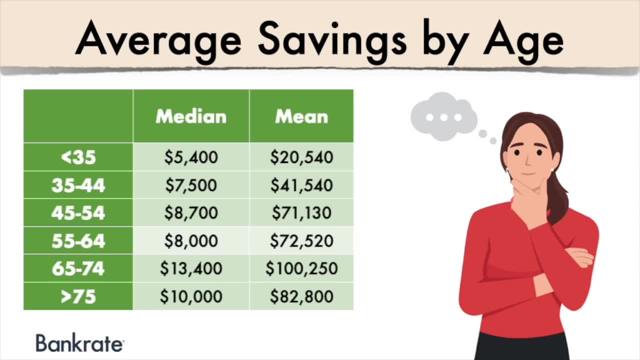 small amounts of outliers with higher account balances. The data includes savings, checkings, money markets and call accounts, as well as prepaid debit cards. So for people 35 and under, the median saving balance is $5,400.. For those 35 to 45, it's $7,500, which is our age group. per day loading next month For those 45 to. 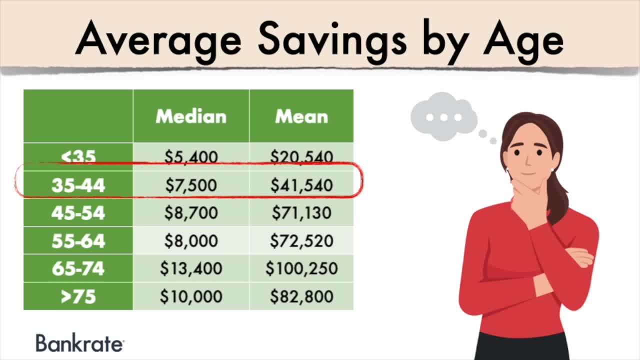 54 years old. the median saving account balance is $8,700.. It drops down to $8,000 for those 55 to 65, and comes back up to about $13,400 for those 65 to 74. And for retirees older than. 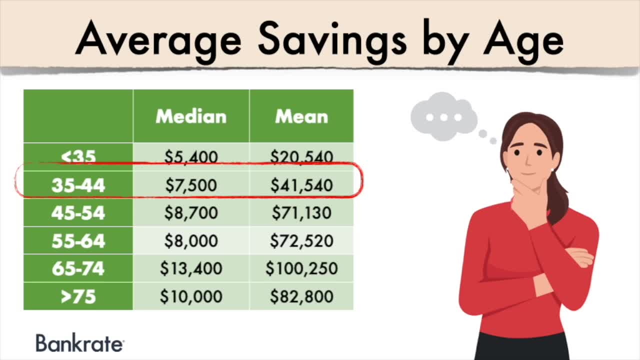 75,. it is at about $10,000.. Things to note: older consumers have had more time to build, advance in their careers and invest in their wealth. It's only natural that they would have higher median account balances than younger generations. But looking at these numbers, 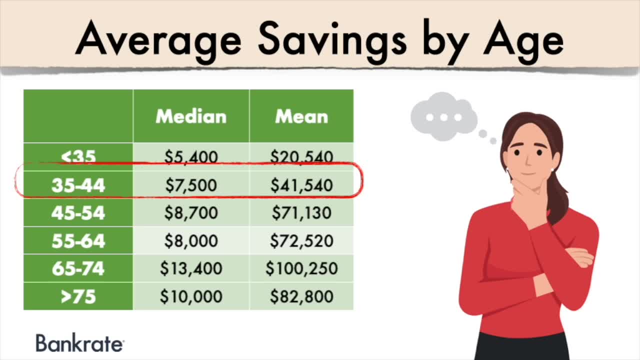 what we can't tell is how many months of security this is for people. One month can be $5,000 for someone, while $5,000 can be two months for another person, And, in general, younger consumers are more likely to be hit by bank account fees, according to Bankrate. 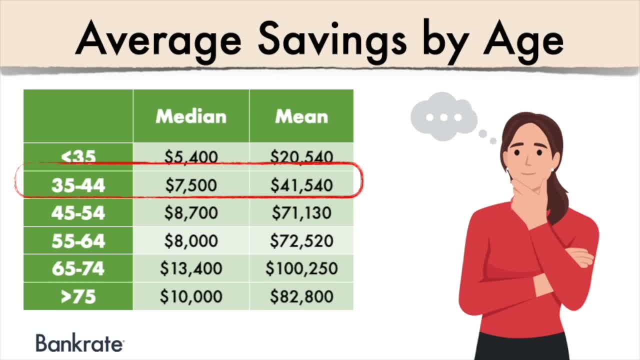 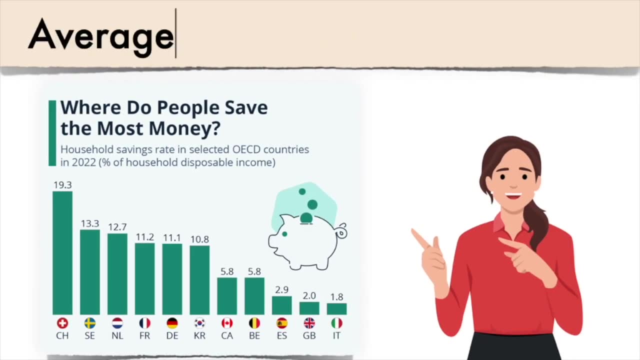 The study found that 46% of Gen Z and 42% of Millennials pay monthly bank fees, compared with only 22% for Gen Xers and 14% on Baby Boomers. So how do you stack up against the average savings account balance in your age group? Comment below: So let's look at how the US stacks up globally. 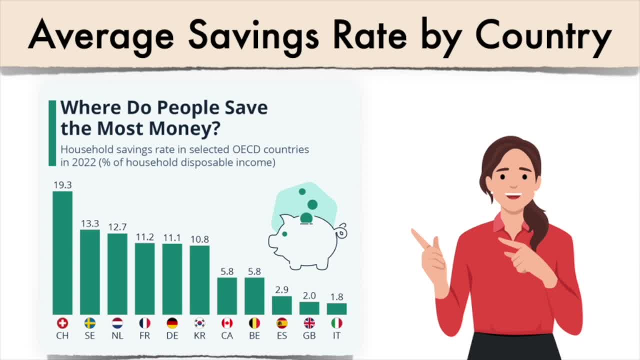 The Organization of Economic Cooperation and Development, the OECD, tracks the household saving rates by country, and the latest data shows citizens in these countries have the highest saving rates per country. So let's look at how the US stacks up globally. The Organization 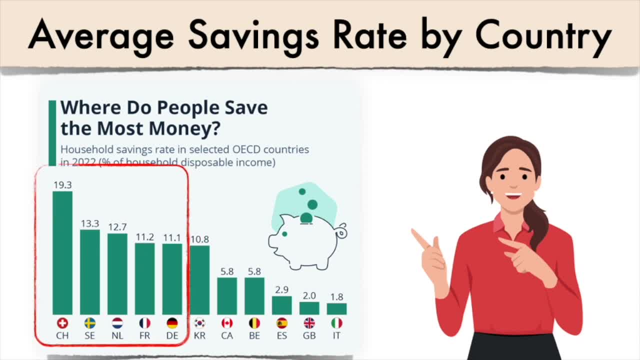 of Economic Cooperation and Development, the OECD, tracks the household saving rates per country. So Switzerland came in at 19.3%, Sweden at 13.3%, the Netherlands at 12.7% and France and Denmark at about 11% respectively. These savings rates are almost three times that of those in America. 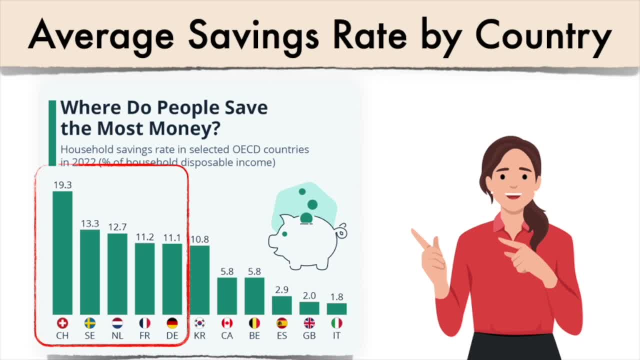 Now, there are many, many factors in play here, such as taxes, income, healthcare, education, childcare, housing and so forth. These comparisons are by no means apples to apples, as all these economic factors do play a role, But it's interesting to analyze what is seen as top savings rates globally. 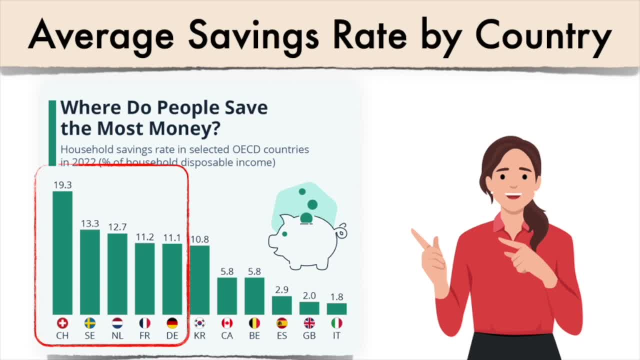 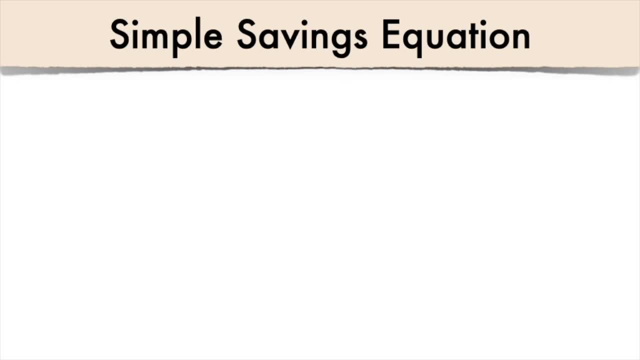 But what ways can you actually increase your savings rate today? Here are three things we did to help us save more. But first let's understand the simple savings equation. So here is an example of a simple savings equation. Savings in sum is taking: 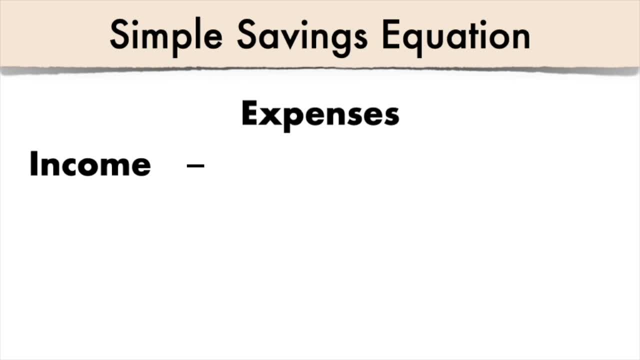 your income minus your expenses and it equals your spread or potential savings. Now your spread or potential savings should increase your income minus your expenses. So let's look at the simple savings equation. You can either focus on increasing your income while maintaining your 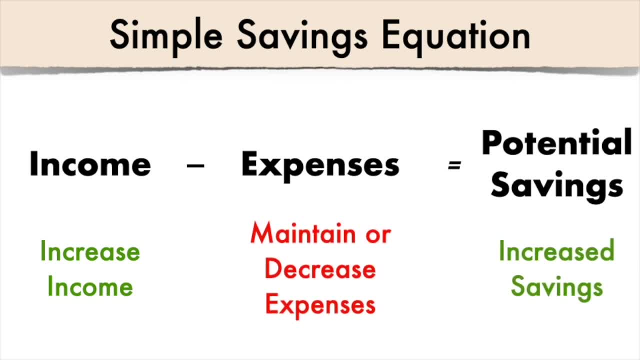 expenses or decreasing your expenses to increase your overall potential savings. Now the equation is making a big first assumption that after you pay your expenses, you still have enough left over to save or spend on anything you would like. I have to keep in mind that many people may still be struggling with this overall and finding ways. 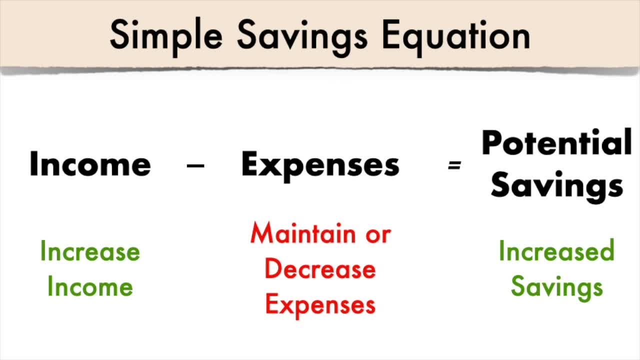 just to meet their minimum expenses For us to start saving more. we initially focused on decreasing our expenses. This is because, if you don't keep your expenses, you'll end up saving more, And when you do that, you are going to end up saving less, And that's because you're not saving as much as you should. 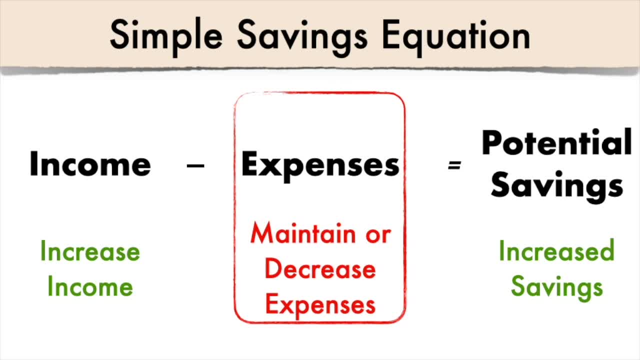 expenses. This seemed like the easiest place to start and helped us to start building a spread between our income and expenses to inevitably save more Once we finally hit our expense baseline. we then focused on increasing our income, which was phase two and what we focused on for the last two and a half years. 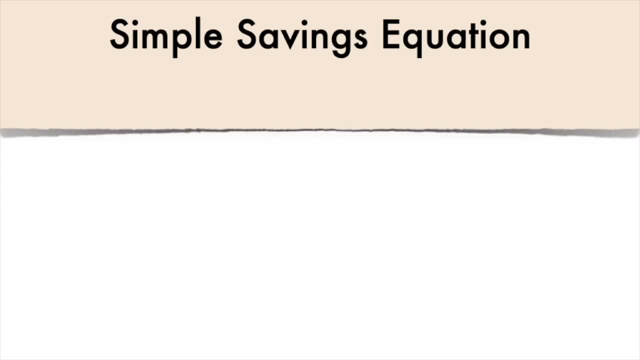 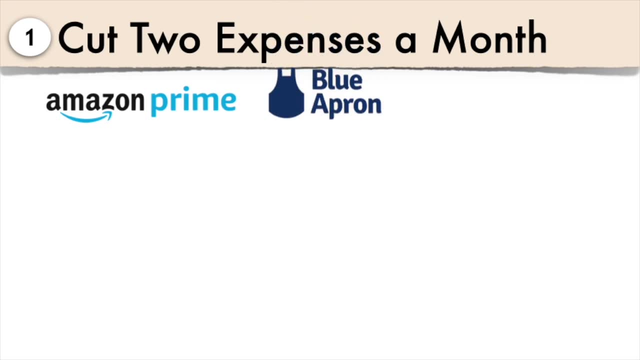 Okay, so here are three things we did to help us save more. The first is obvious: We cut our expenses, but we did it slowly. We didn't make any drastic changes like cutting our expenses by 50% in one month. We wanted the transition to be sustainable and gradual, but in the end this helped us. 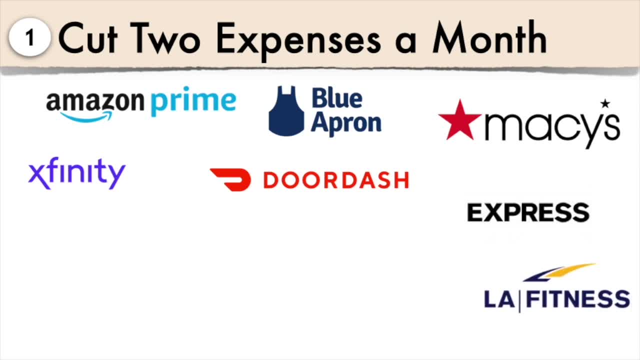 quote. unquote- find more dollars in our budget. We focused on cutting two expenses a month or eliminate discretionary spending in areas that we didn't need. Some months we decreased three to four expenses and others it was just one, but on average we eliminated about two key expenses over a year. 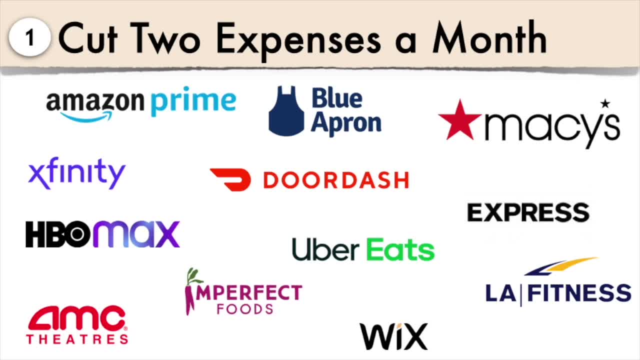 Here are the list of things we eliminated. The biggest was getting rid of Amazon Prime, and you're probably thinking well that membership is just about $15 a month, But it wasn't the cost. It wasn't the cost of the membership we eliminated, but the excessive shopping that went with. 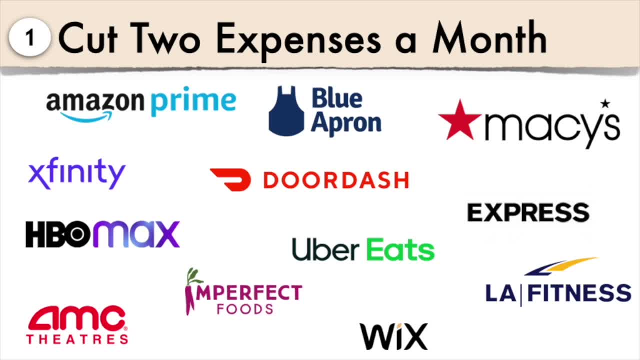 it. We- or shall I say I- had an Amazon addiction and we used to live next to a DC, so items came same day all the time. Removing Prime helped mitigate and almost eliminate our Amazon spending. When we needed an item, we did it the old fashioned way. 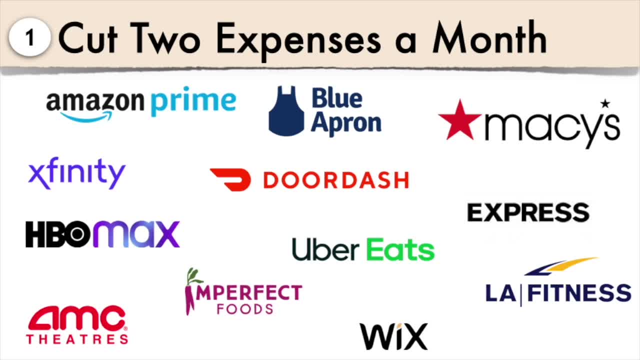 We went to the store and we got it. I also found that many items we were buying were not necessarily the lowest cost on Amazon, as there are many, many resellers on that site. Another big expense we cut was food delivery services. We don't use DoorDash or Uber Eats or Grubhub at all. 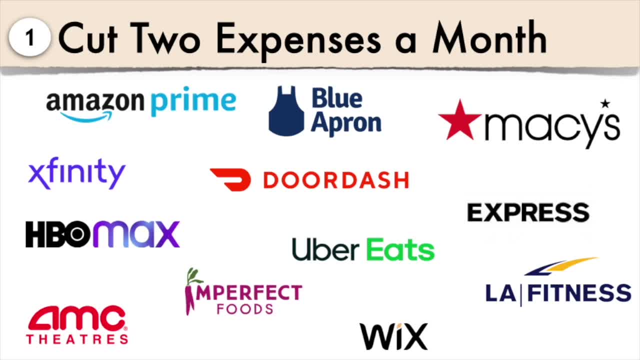 If we are doing takeout, we call the restaurant or use their online portal and we order from there. This has saved us a lot and helped us decrease our spending on takeout. The only time I may use a delivery service is on a work trip, when it's expense to the. 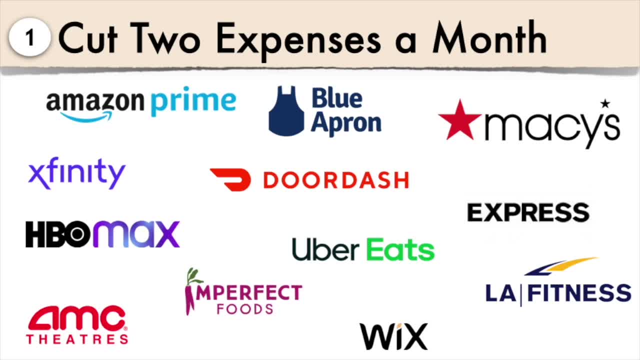 company. Another expense we got rid of was getting rid of our LA Fitness membership. Now I love the gym. I still love it, But after COVID I found pleasure in working out at home and working out alongside YouTube videos. Today at our house, we have an elliptical ropes, boxing bags, weights, weight machine. 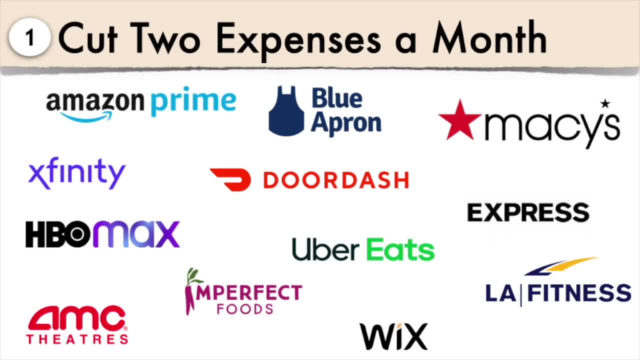 ab roller and mats in our home And for most of these items we got them for free on Facebook Marketplace. Workout items are a pain to move with, so many people ought to leave them behind when they switch to a new home. That's when we swoop in and get it for free. 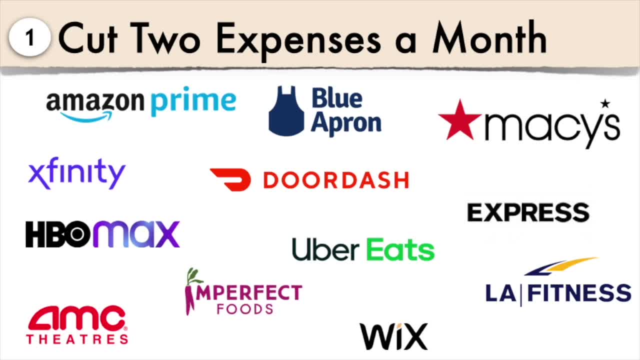 I get my gym fixes on days I travel for work. I spend a good chunk of time in the gym when I'm there, But if we do move, I would like to get a treadmill one way or the other. I am always reviewing our budget to see where we can find cuts. 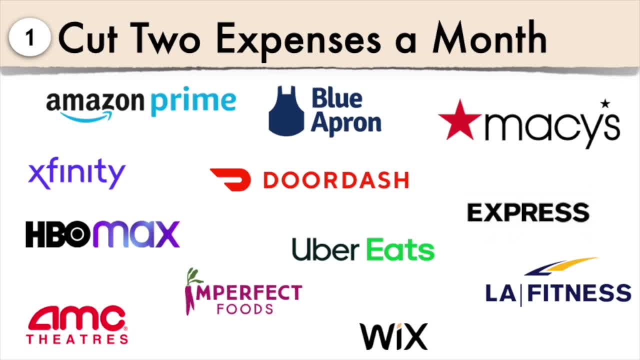 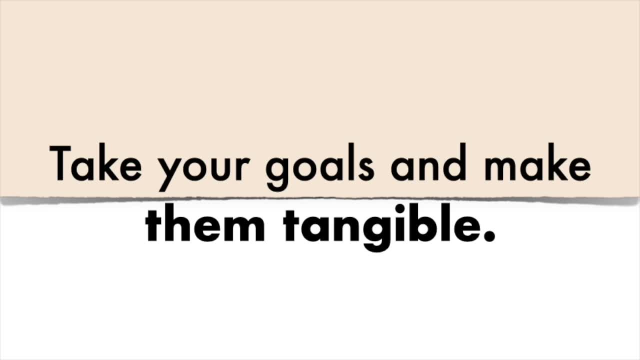 Right now, I feel like we're in a good place, especially after eliminating all of these expenses here. Now take your goals and make them tangible. The biggest mistake or problem I see with savings is the goal seems too big. I want to save $25,000, but how? 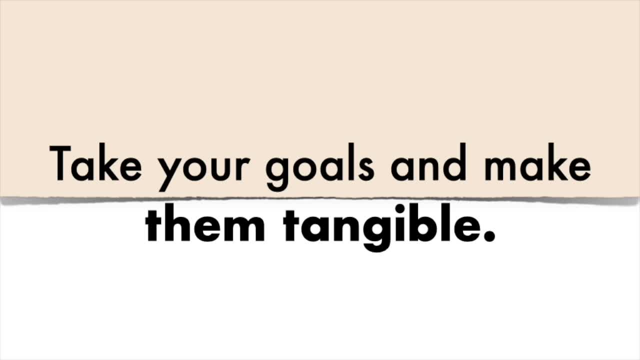 What steps are needed to get there. I always find ways to break down our goals into small steps. I want to save $100,000 in one year, but I know that isn't possible due to many factors—mainly our income. So we took our emergency fund goal and broke it down into the years and then into months. 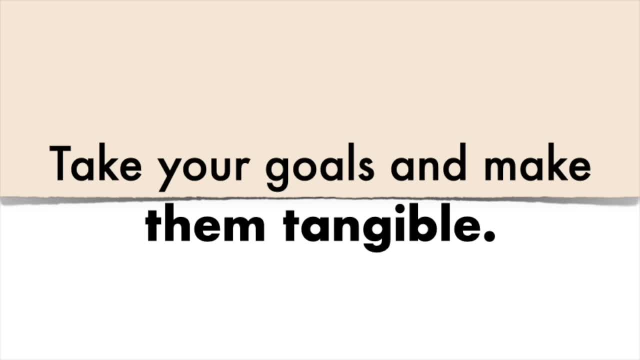 to be able to make it more tangible. It's going to take us four years to get to our goal, and that's okay. We will take the measurable steps we outline and get there one way or another. We finally began to review our expenses during COVID. 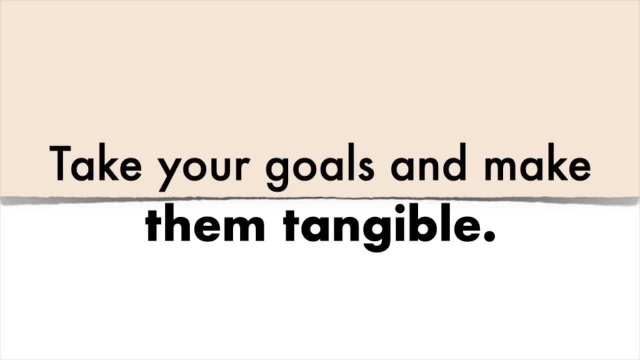 The first thing we did was review our expenses. The hard truth about our expenses overall is that we were living to keep up with others. We were living in a large, trendy, hip city and wanted to keep our lifestyle to mimic those around us. 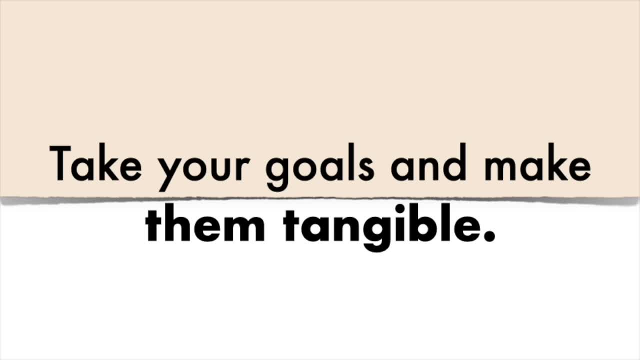 We did what our co-workers did: We went out, We dined out all weekend, We spent and spent and spent to maintain an image that was keeping us broke. It's not easy, but we had to take a moment and check ourselves. 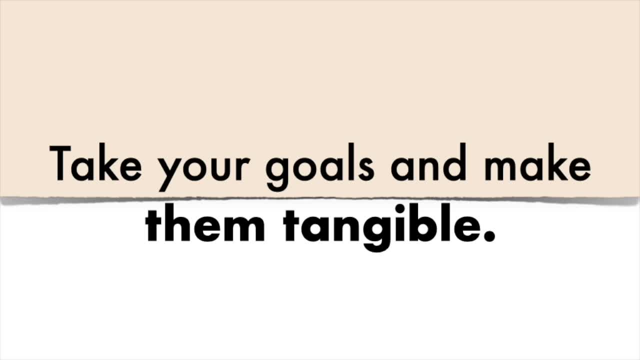 During COVID we had the time to do that and it finally clicked for us. I know when talking about savings and building an emergency fund, we always think about the direct monetary option. We were not only re-evaluating our expenses, but we re-evaluated what we were consuming. 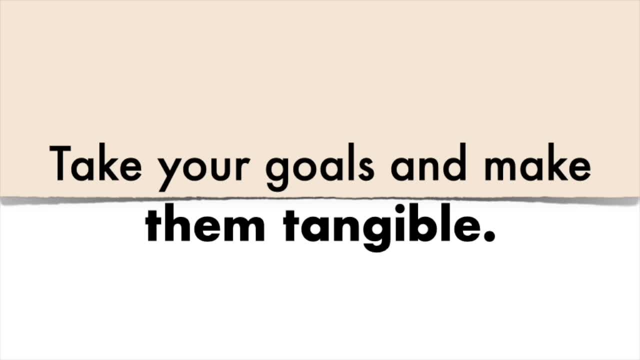 watching, reading, listening to, putting in our minds and who we were hanging out with as well. Did we surround ourselves with like-minded people, or were our friends also keeping us broke? We also re-evaluated our time. Where or what were we spending our time on and what was the cost, including opportunity? 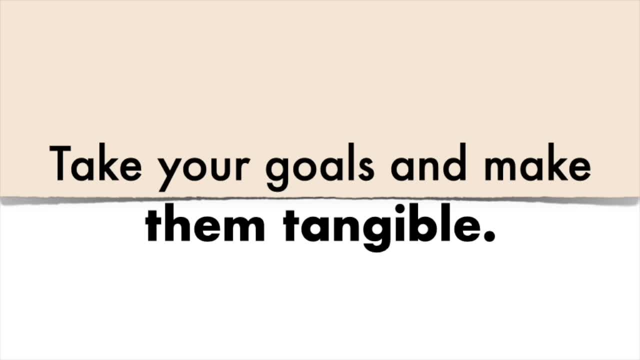 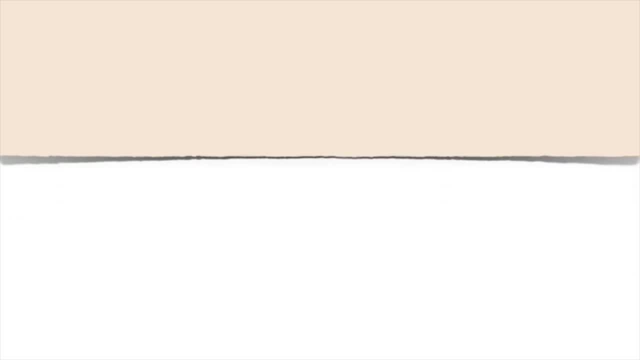 costs associated with these events. Sometimes, these non-monetary sections outside of your budget are the ones that make you feel like you can't afford to spend the money you're saving. They can impact your spending as well, and we unfortunately learned that the hard way. 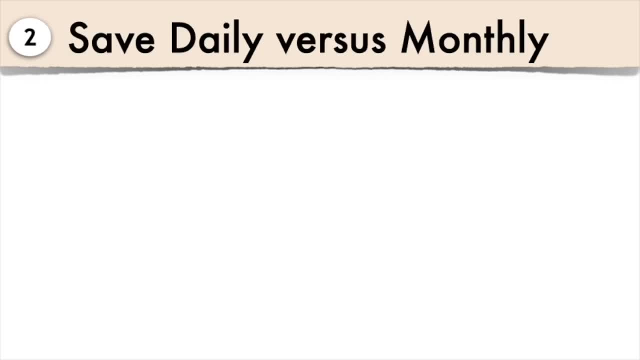 So, number two: a great way to make your goals more tangible is to break them down. We opted to save daily versus monthly early in our savings journey. Now we did this electronically, but I've seen this done with cash envelopes as well. 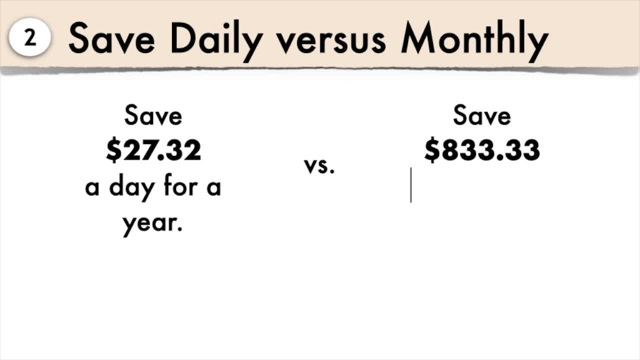 Our first goal was to get $10,000 saved. At this time we never had our savings higher than about $8,000 at the most, and that was usually due to bonuses. So we focused on saving about $27.32 a day for a year to help us get to that $10,000. 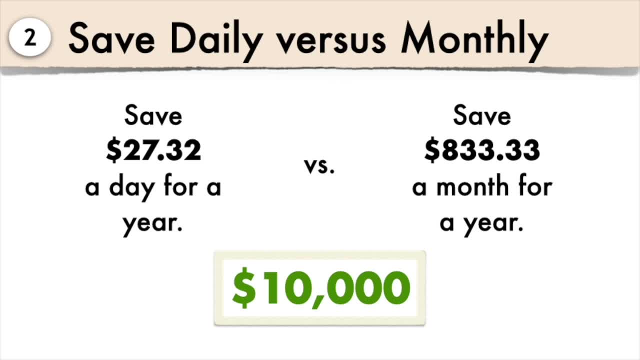 mark. I would simply transfer about $27 to our savings account from our check-ins each day. Now this was much less scary mentally than saving $833 a month. What this did was also curb our daily spending. That $27.32 would have gone to a quick chipotle meal or a quick one to the dry cleaners for. 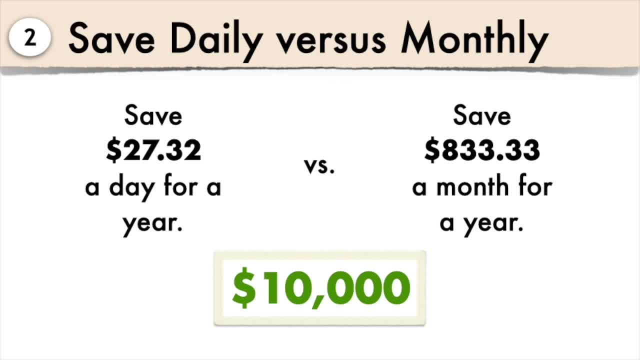 a shirt I didn't need clean. So we decided to save $10,000, and save $2.73 a day for a year, versus saving $83 a month. But if $10,000 is too much, start with $1,000, using the same concept. 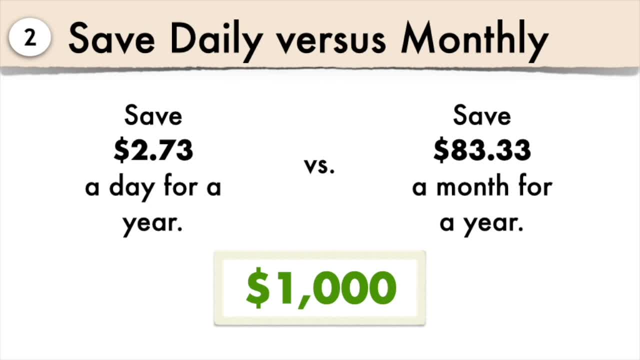 Save $2.73 a day for a year, versus saving $83 a month. This is taking your overall goal and breaking it down into bite-sized steps. $1,000 might seem like a lot, but $2.73 a day is approachable. 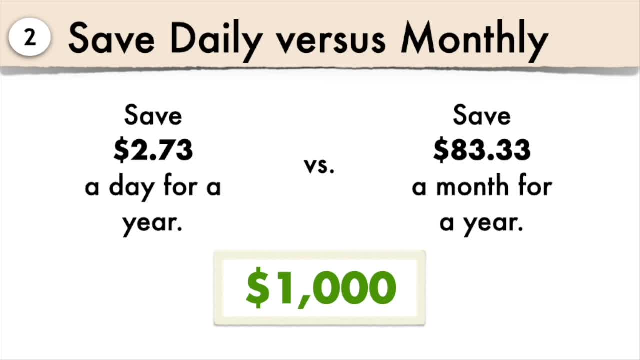 I'm not sure we can get for $2.73 today, maybe gas or a lotto ticket or one item at the dollar store. I'm not sure we can get for $2.73 a day, but I'm not sure we can get for $2.73 a month. 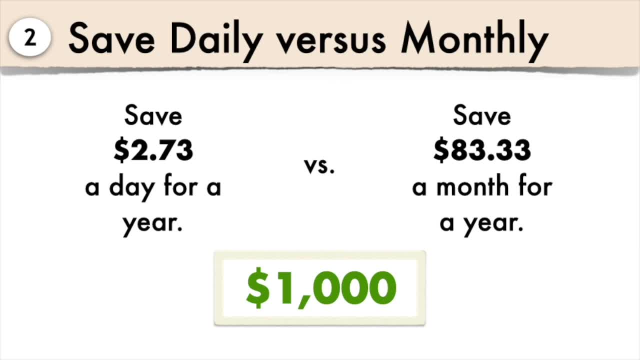 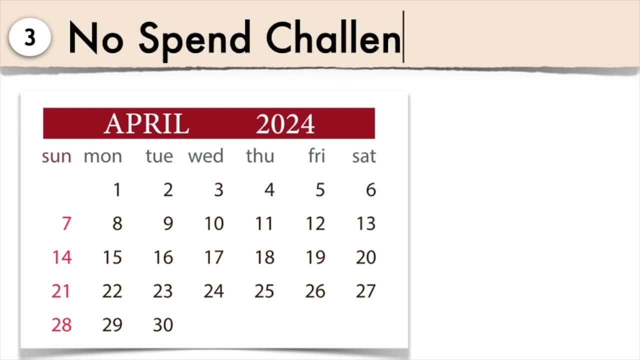 Now, if daily is too much, focus on weekly, These small shifts helps us get into the habit of saving. Okay, number three: we did no-spend challenges. It's very simple: We allocated days where we wouldn't spend money at all. 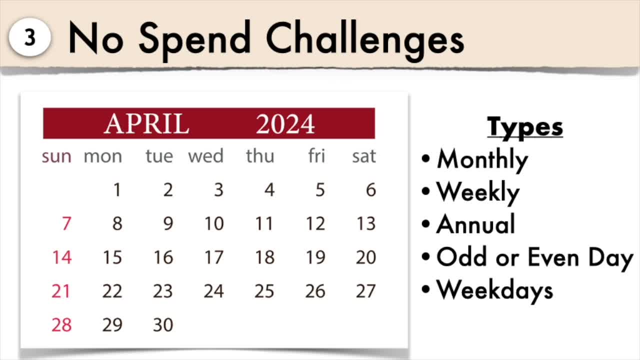 Now there are exceptions. If there was an emergency or health issue that arose, like someone got sick and we needed baby time, then of course we would spend the money as needed. But a no-spend challenge allows you to restrict your non-essential spending. 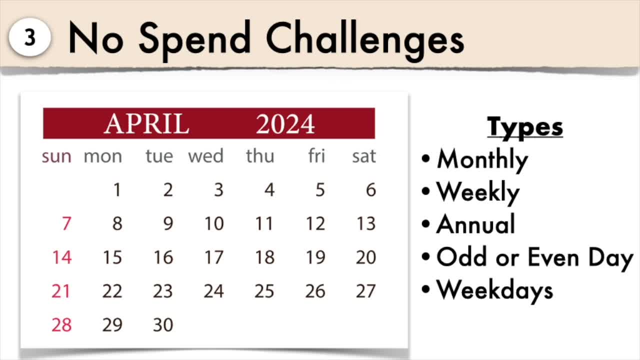 I find these challenges to be very helpful when it comes to spending, Because first it felt like a game. We had printouts and marked it up as we went. The first one we did was an odd-day only challenge, where we only spent money on odd-days. 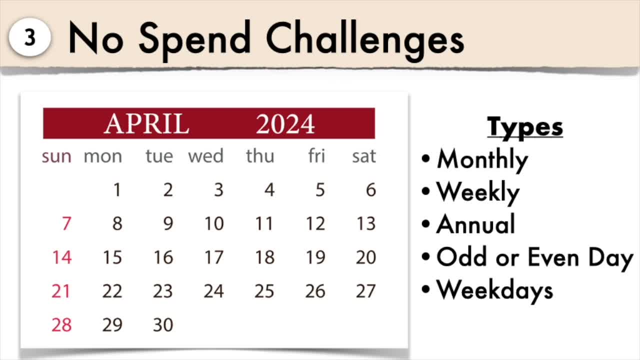 We did a no-spend month as well, where we only spent money on items we needed for that month. That meant no takeout, no new Nike Air Maxes, no new plans or what other items we would have spent our money on that month. 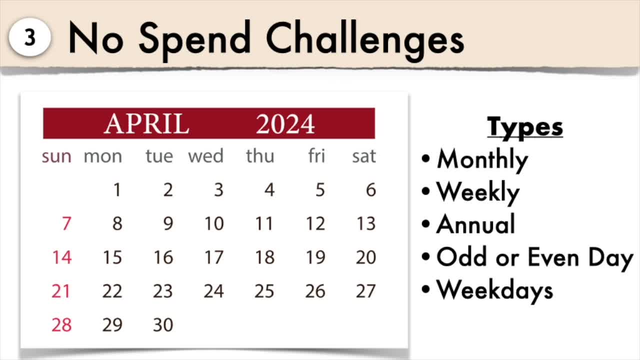 During COVID. we couldn't spend at the usual places. We couldn't go out to eat. We couldn't go to the movies or the bowling alley. We couldn't go to the movies or the bowling alley. We couldn't go out to the movies or the bowling alley. 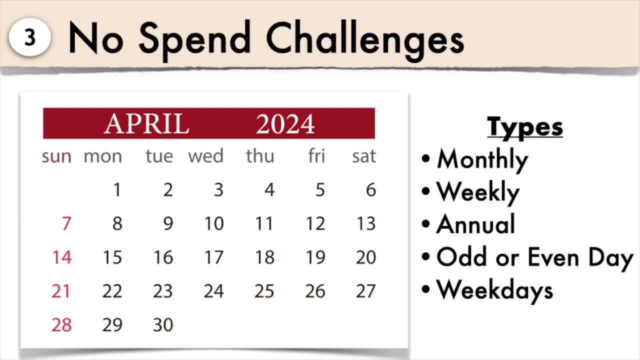 bowling alley, we couldn't spend money on anything that was not deemed essential. The principle or the idea is the same for these no-spend challenges: Start with a set few days, then move into weeks, months or even seasons, but find a block that works for you. Now I've seen this done in a 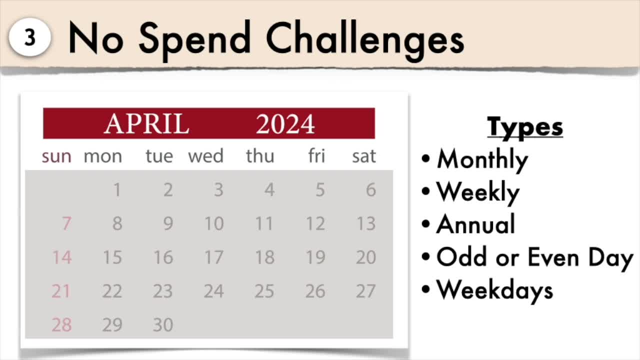 simple, tangible way- and I've seen it done in a very extreme way as well- Find the right balance that works for you. Our no-spend challenges helped us get the ball rolling on savings overall, So here's a look into our savings accounts. with Capital One, Most of our money is in our 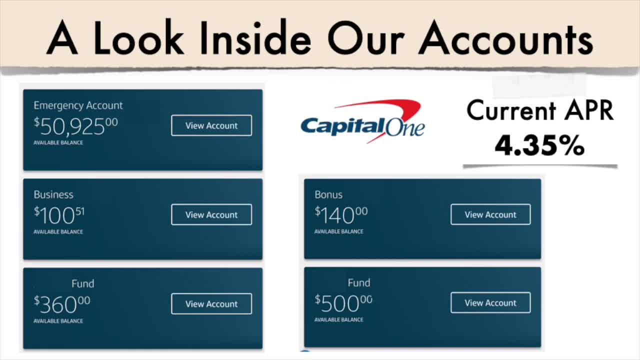 emergency funds, but we do have a few other savings accounts. We have a small business account so I can easily track our business expenses. We then have an account for each child and that's where we put their birthday or holiday money prior to sending it to their 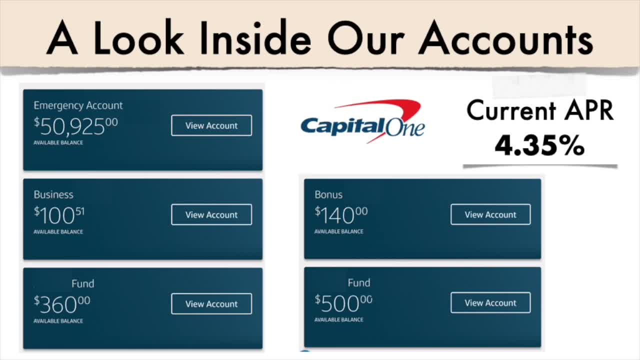 UTMA accounts And then new this year is a bonus account. I put all of our bonus income here so I can track it easily, but it is also included in our total budget. Right now, Capital One has an APR of about $1,000.. So that's a lot of money. Now, Capital One has an APR of about $1,000. 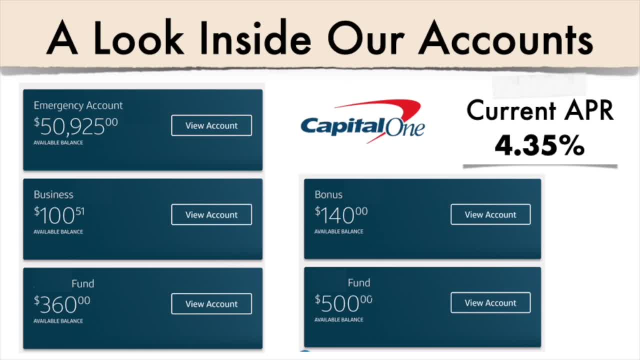 So that's about 4.35%, And I'm wondering if it makes sense to move our money to another account with a higher rate, as I just noticed that even Vanguard has a cash account option with an even higher APR. The annoying thing is that all of our automatic transfers are already tied to these. 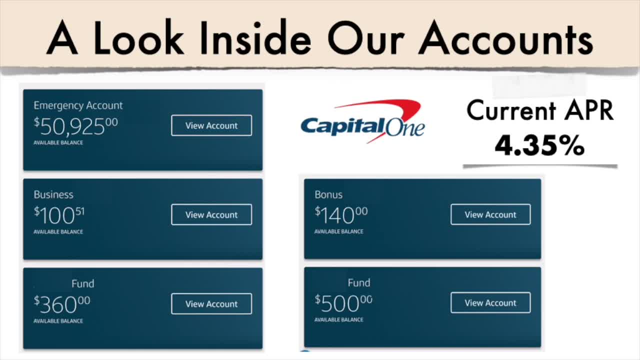 accounts. so change means rework on my end And if you're new here, my goal is always to keep things simple. Also, there is this rhetoric in the market about rates dropping, so I might just wait it out for a bit. Anyways, we have ways to go to get to our account, to that one-year mark for our emergency. 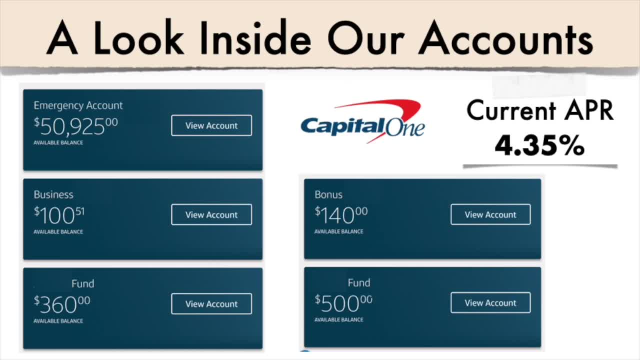 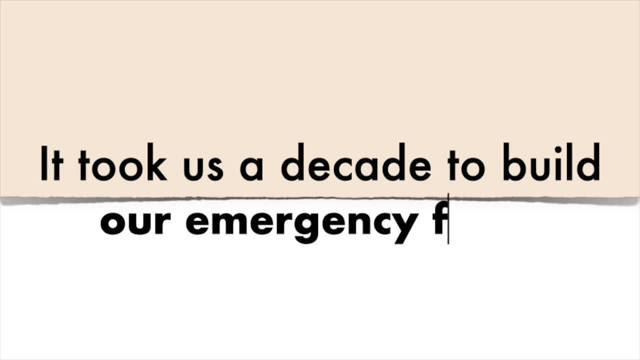 fund, but we're happy with our money, So let's get started. Progress so far- All the minor savings, changes, challenges and expense reviews- is definitely paying off. But it took us a decade to build our emergency fund, to build our accounts to $50,000. 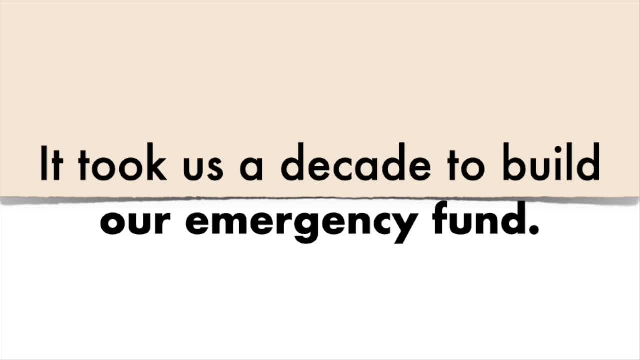 Now I'm not sure if 10 years is normal or not, but we finally got to a solid six-month emergency fund. Cutting expenses, building tangible habits and getting into the habit of spending less helped us reach our goals. But we didn't stop there. We did focus on one side of the equation. 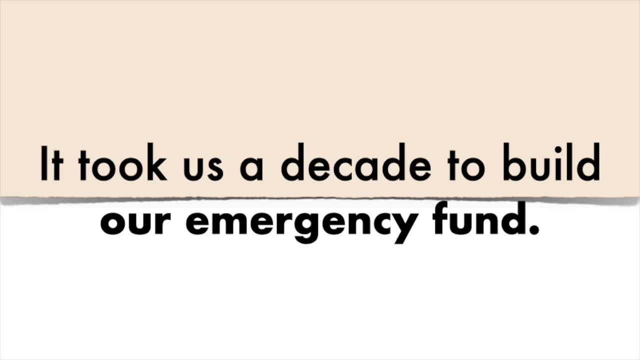 expenses but shifted to the other side. Those two coupled together helped us expedite our savings goal And, honestly, I think income growth was the true catalyst. Today, I feel we hit our core or base expenses. I don't see us cutting out. 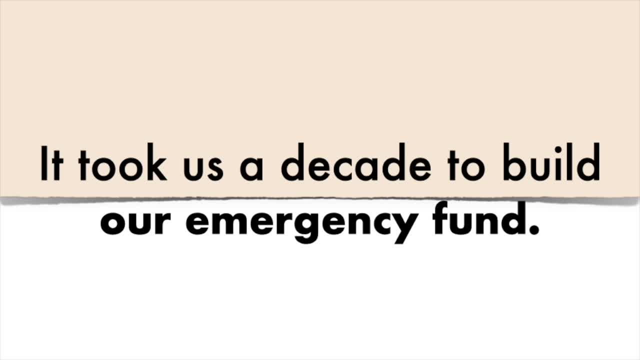 more or anything else without diminishing our current way of life. There is a balance, and I think we found that right balance. Right now our savings rate is about 29% and this month we're tracking towards 32%, which is exactly where we expected to be for the year. But I'm lucky to have 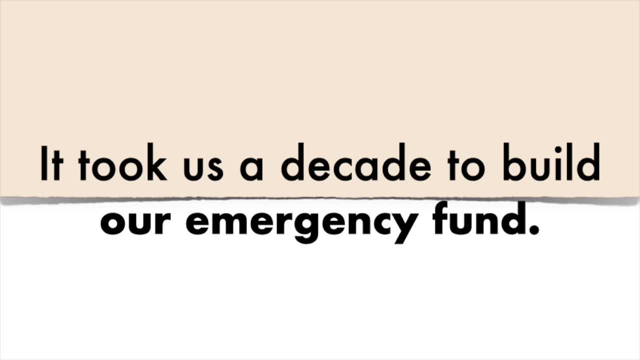 that balance and I'm happy to be able to do what I want to do, and I'm happy to be able to do what I want to do. He just doesn't find joy in spending and is very frugal overall. He also is very handy and can fix. 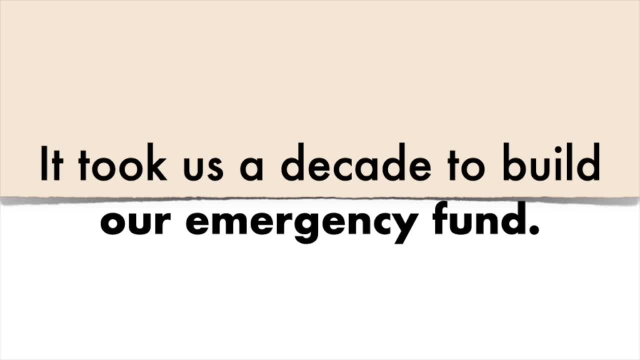 or refurbish almost anything in our home. Having a partner with the similar or same money mindset also helped us reach our goals better. I wouldn't be here without him. Sometimes, almost all the time, it's the non-monetary choices and changes that will have the biggest, if not largest impact.